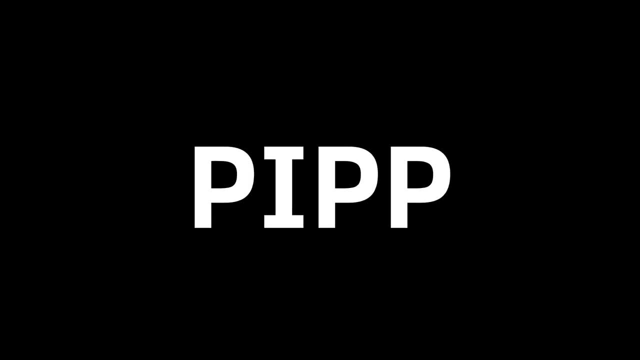 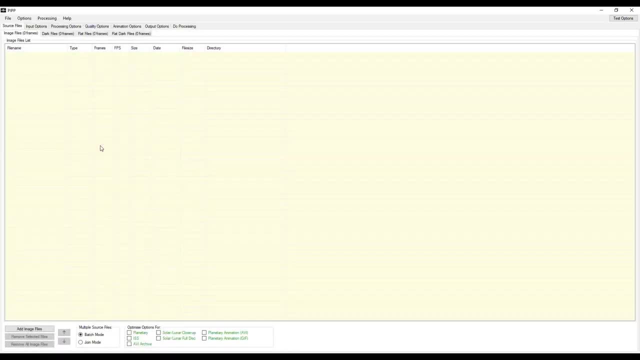 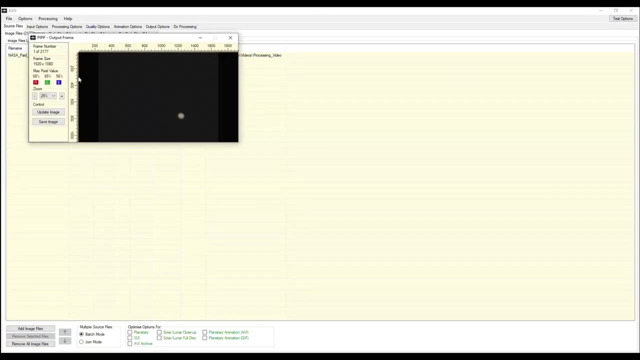 in the description, and we are going to start with Pip, Pip, Yes, Pip. This program has a simple interface, so it's pretty impossible to get lost in its features. For a start, you need to add the recorded video with the planet to the program and it will appear in a separate 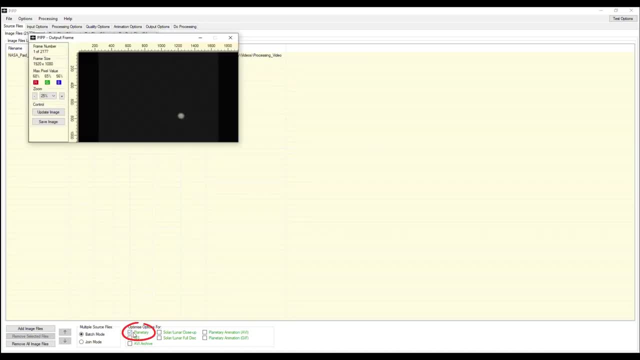 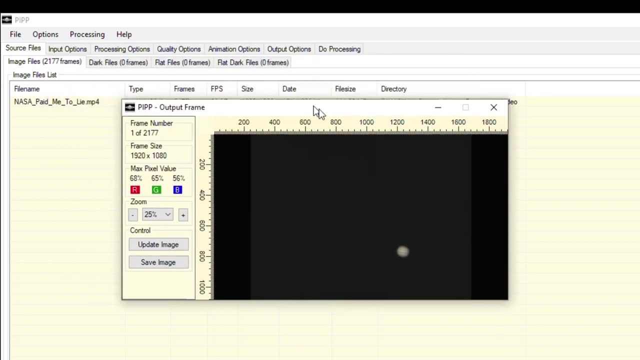 window. Then you choose the option Planetary to place Jupiter in the center of the video. However, there is lots of empty space around the planet. You can click on the tab Processing Options and change the size of the window, just don't crop the planet itself. 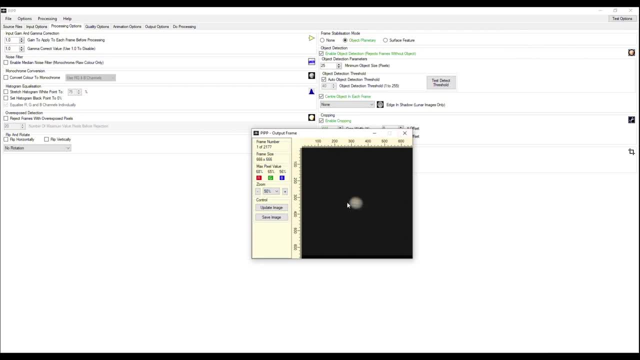 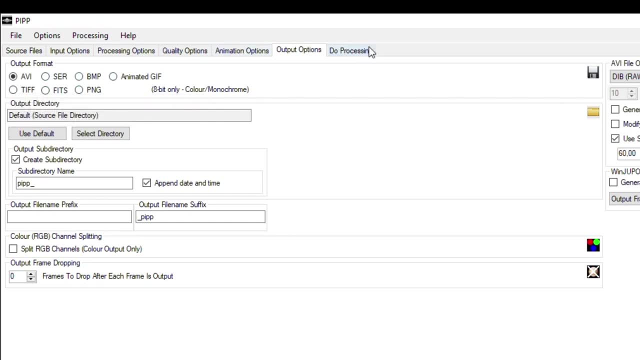 If this video was useful, please like it, share it with your friends and subscribe to our channel. Thanks, Bye-bye. size satisfies. you go further to output options and check if the file format is AVI. This is important. Finally, click do processing and then start processing Now. 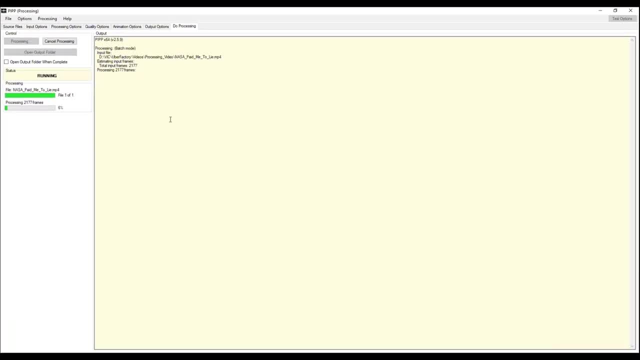 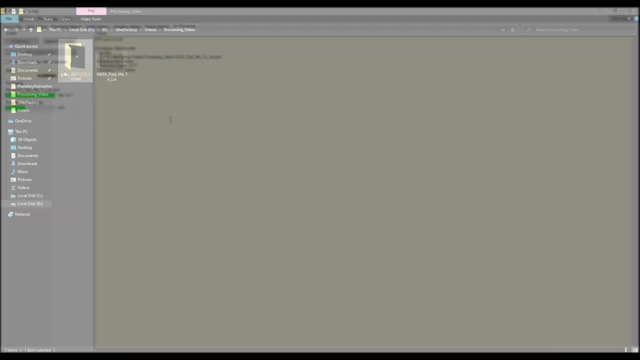 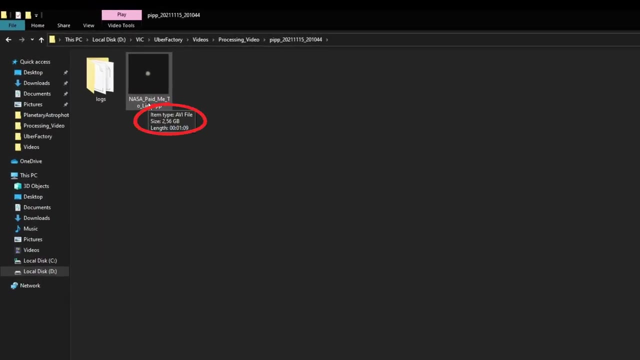 you just have to wait until pip edits all frames, and in my case it's 2177 frames. Next the program will open a folder with a cropped clip, and don't worry if your file size is several gigabytes. that's pretty normal. Now the 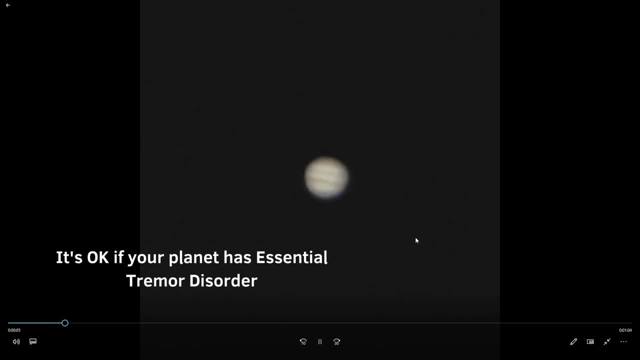 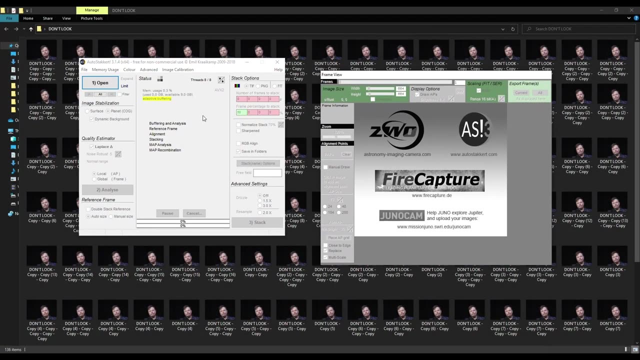 planet is located right in the center of the video. so it's time to use the next software called AutoStackert. As you see, AutoStackert has many very interesting features as well, but we will use only a few of them First of all. 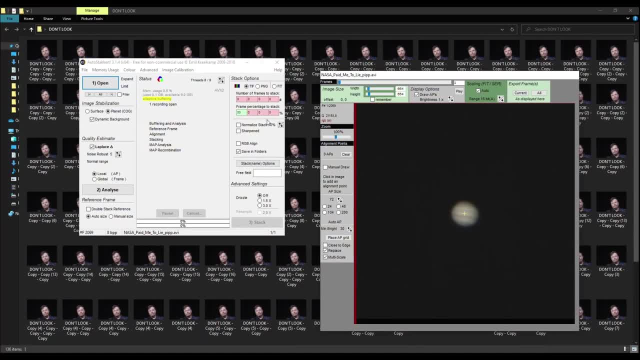 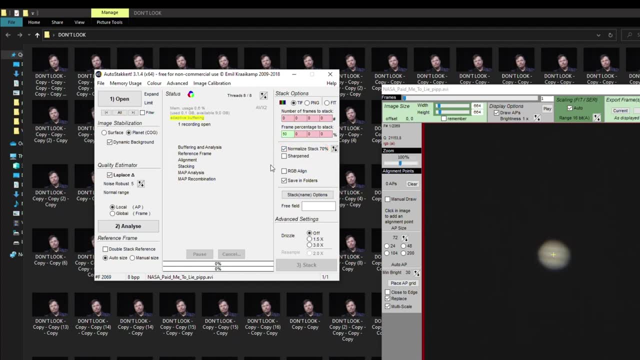 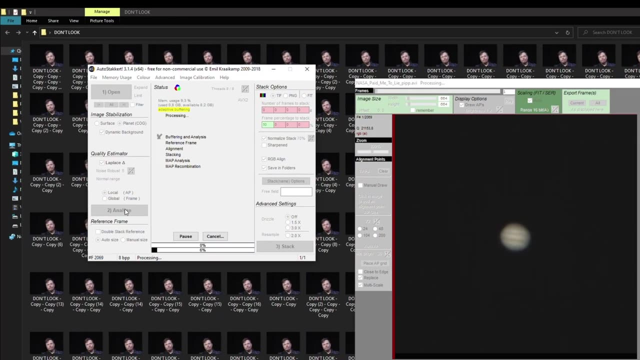 click open and find a processed clip on your PC. Put a tick on the item planet and normalize stack 75. to normalize the brightness, Choose AutoStackert, Then choose RGB align in order to reduce the atmospheric distortion that affected the image, and click analyze. After successfully analyzing all frames, the 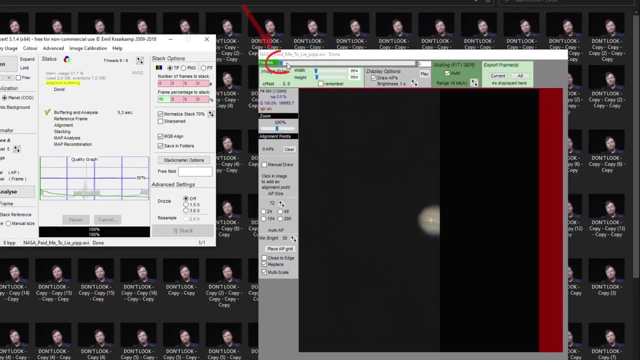 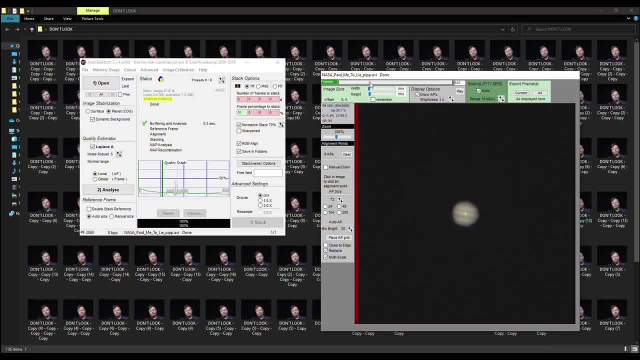 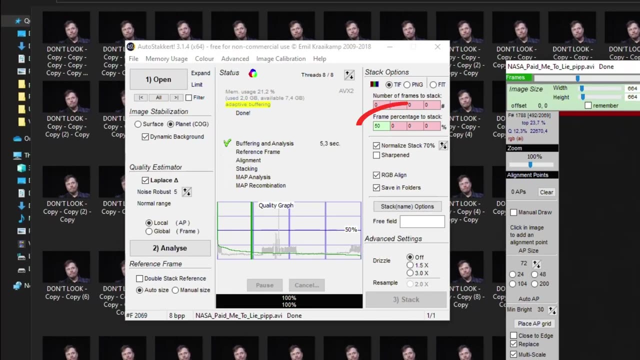 program will sort them by quality. You can move this slider and see how the frames change, from the best ones on the left and the most disgusting ones on the right Among them. you need to find a decent picture- not an ideal one- that doesn't look blurry. Now it's time to indicate the percentage of frames that 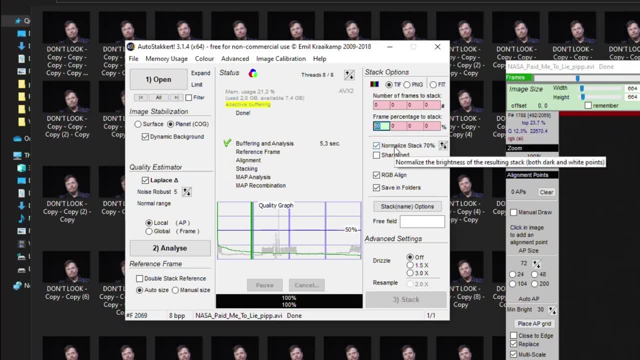 you want to stack. The amount frequently depends on the atmospheric conditions that were during the shooting. If the quality of the video is high and the scene was pretty good, then you can stack from 33 to 50 percent of all frames, but if the recorded planet 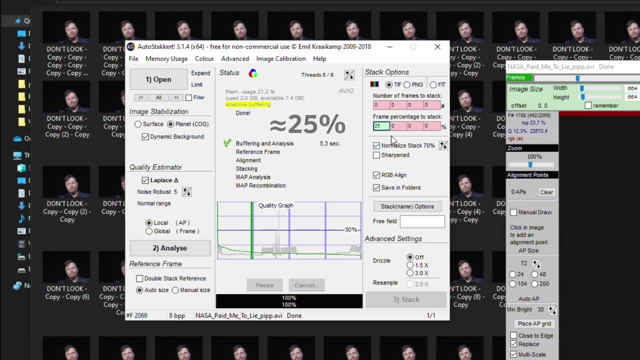 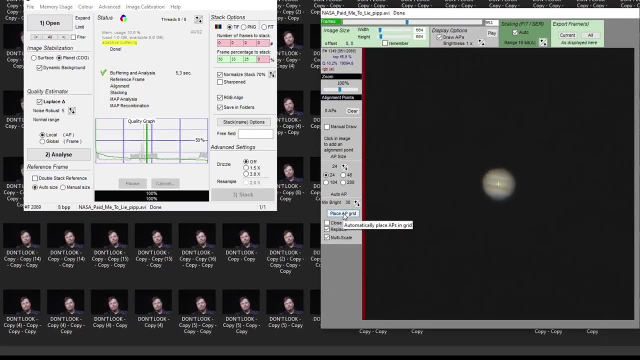 looks blurry, indicate a smaller number. You can actually tell the program to have several options like 50,, 33 and 25 percent. Next, we need to assist AutoStackert in successfully stacking all frames by clicking Place AP Grid. It'll create many alignment points. 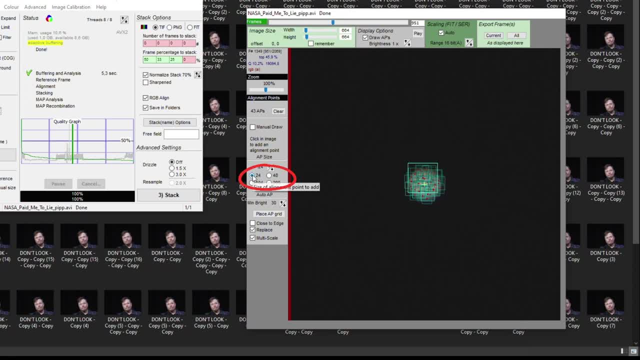 around the planet and you can change their size. here I recommend sticking to 24.. In case the amount of boxes does not satisfy you, you can remove some of them with the right mouse click or add new ones with the left mouse click. Do not. 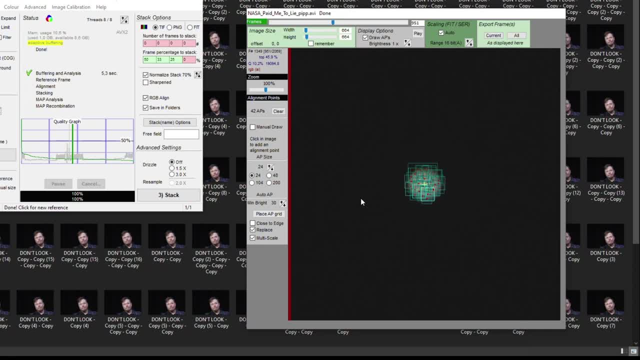 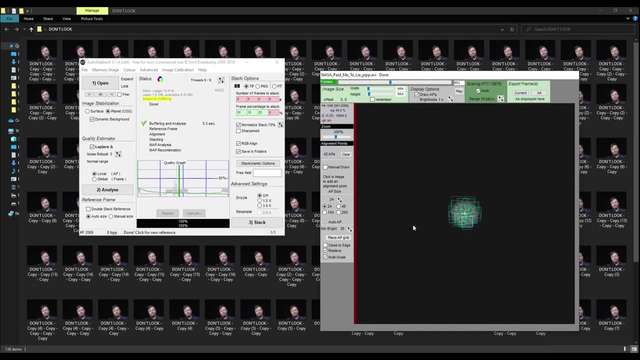 forget to set points on moves that are in the frame. If the recorded planet is quite big, like Jupiter, then that's all you need to do, But if the planet is small like Uranus, then we don't need so many points. 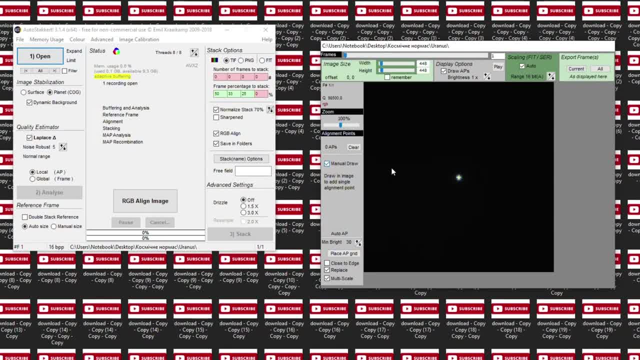 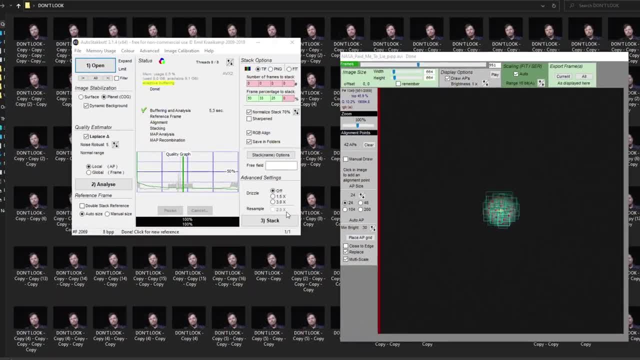 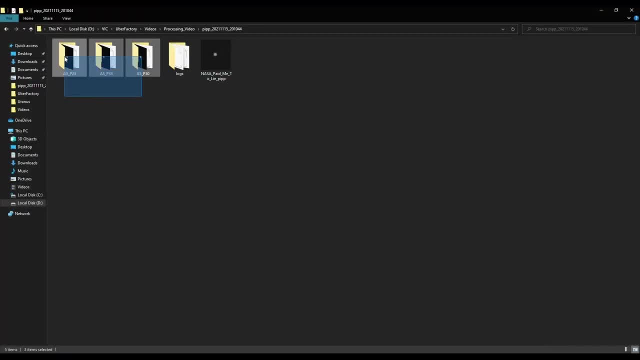 for such a small object. Press the button Manual, Draw, make a left mouse click and place the planet right in the center of this box. Finally, you click Stack and simply wait. It takes several minutes to process all frames. After that you'll get. 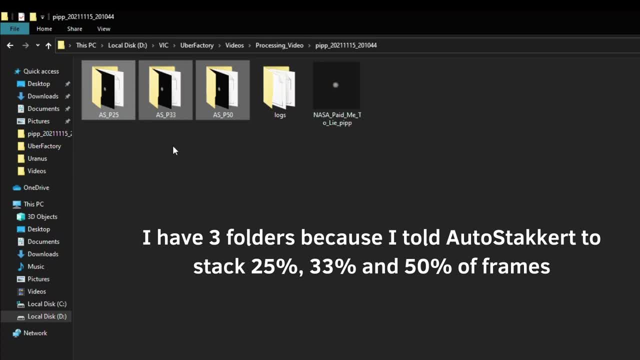 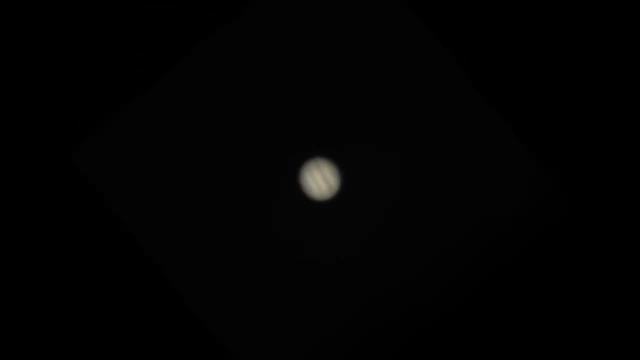 your processed image in the folder where the pip file is located. As you see, it's still quite a blurry picture, so the final editing will be made in the last program, called RegiStack 6.. By the way, when you visit their website, you need to: 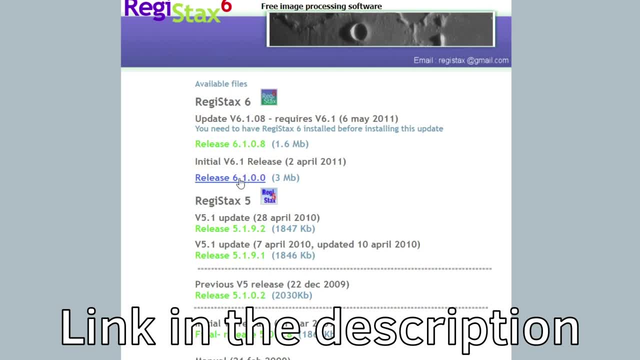 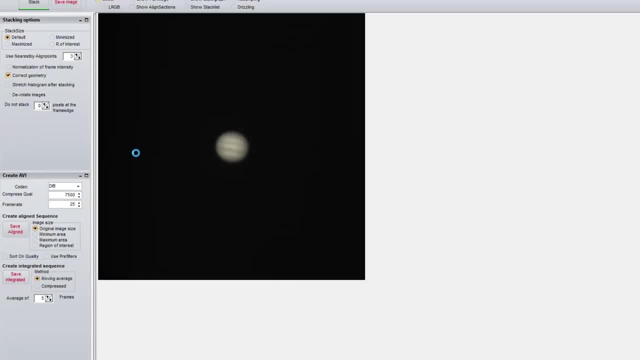 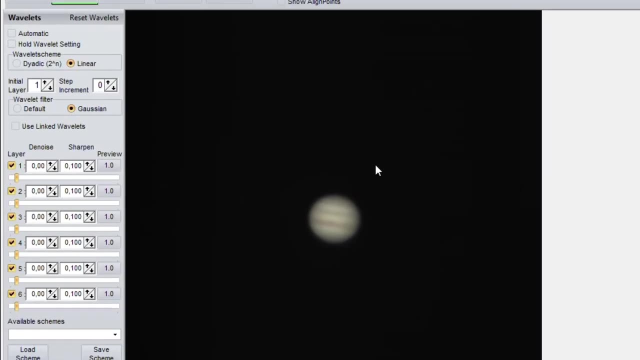 download this version of RegiStacks, since the other ones are simply updates. After opening, you press the button Select, find your magnificent file and choose it. Then you go to the tab wavelet to do the final editing of your planet, where you will need these settings. on the left, I often choose the 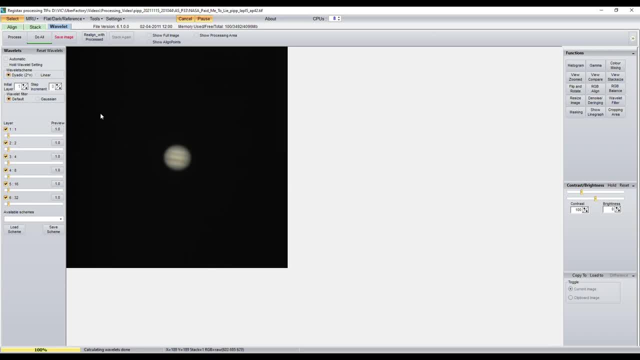 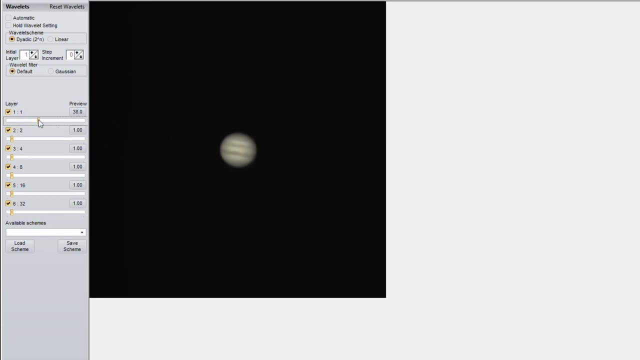 the dyadic wavelet scheme and a default filter, but these settings depend on a planet, so you can experiment by using different schemes To increase the quality of the image. you need to move these sliders below the filters. I never use the first one because it frequently adds unnecessary grain to the image and I